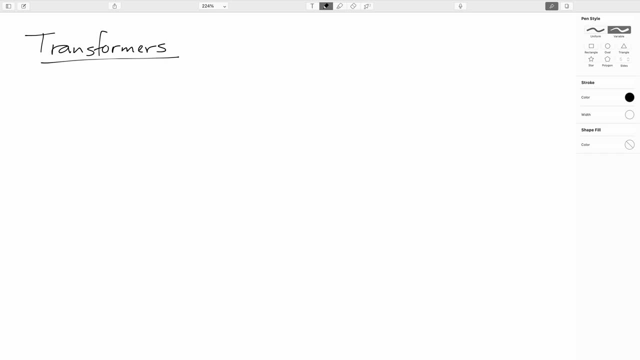 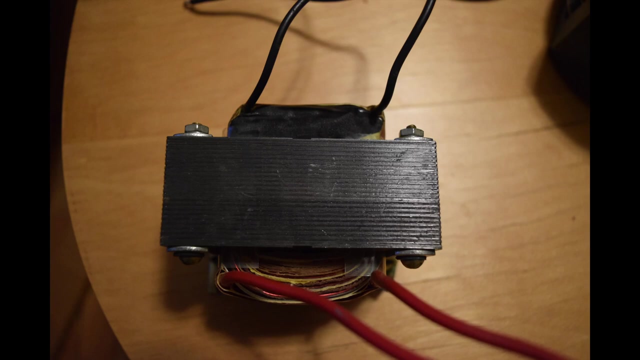 In the last video we introduced AC circuits and I mentioned that one of the reasons why AC electricity was preferred for power transmission was a uniquely AC device called a transformer. So this is a not terribly big transformer, but it is a transformer. The red wires here: 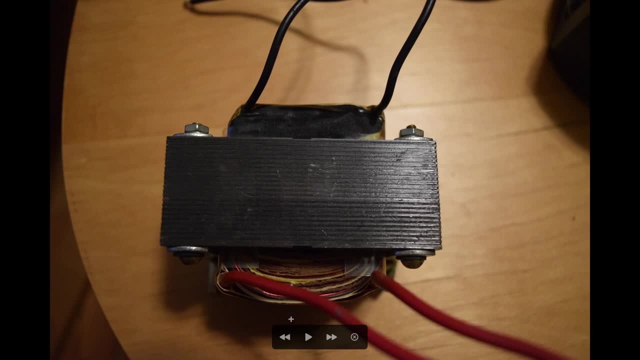 are connected to one coil of wire, going around like this, and the black leads are connected to another coil. They are going around a common iron core. You can't see that here because it's in the way, but there's an iron core going all the way through and then it wraps around in order to help. 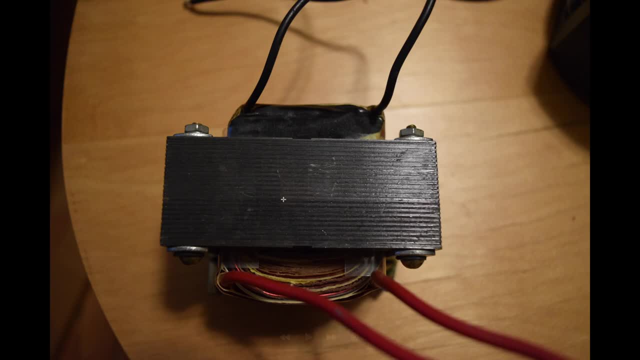 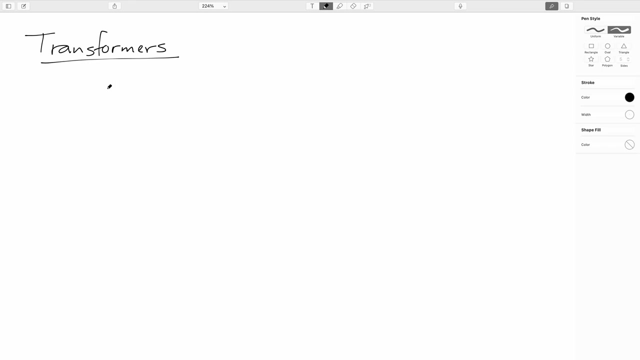 guide the magnetic field lines going through the area. Now, there's no electrical connection whatsoever between the two coils, It's purely, they purely share a magnetic field. So what does this do for us? Well, the idea here is that, by Faraday's law of induction, if we look at the output of the 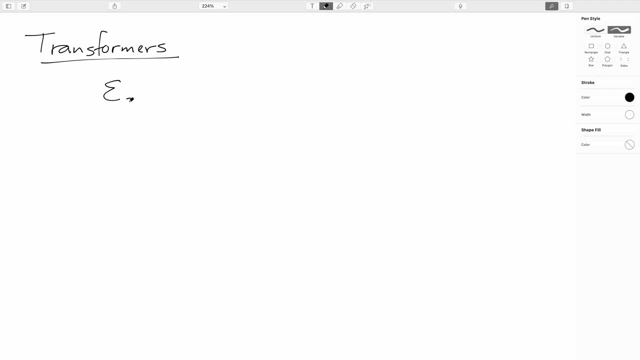 transformer, which we usually call the secondary coil, that will be equal to minus the number of turns. Now, the number of turns in that secondary coil times the time rate of change of the magnetic flux going through it, And if i divide by the emf across the primary coil. 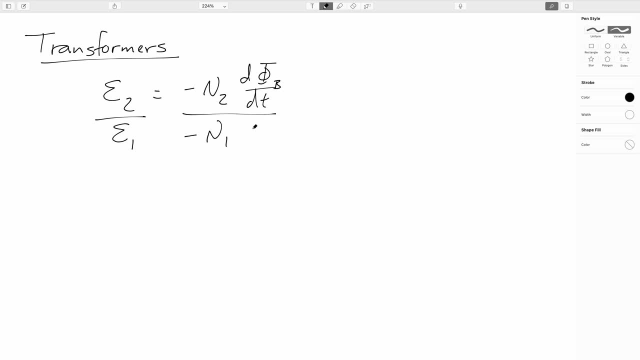 by Faraday's law of induction, it will be minus N1, d phi b dt. Well, the minus signs and the d phi b dt's cancel out, and what we get is this: is that the ratio of the ems, which would be the voltage across the secondary to the voltage across, 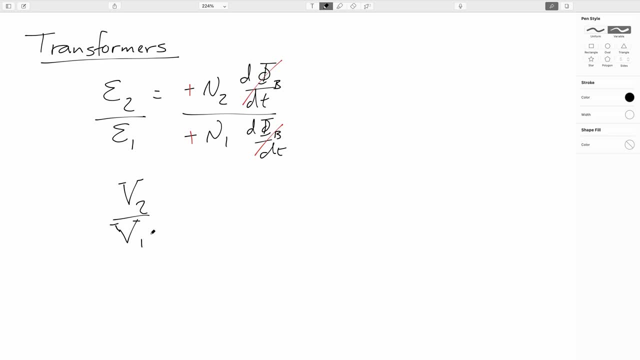 the primary. so just the primary is where you're, you're going in, and the secondary is where you're going out- is equal to the ratio of the number of turns. so what this does is, let's say you have 2000 churns on the secondary and 200 churns on the primary. if you had 110 volts going into the 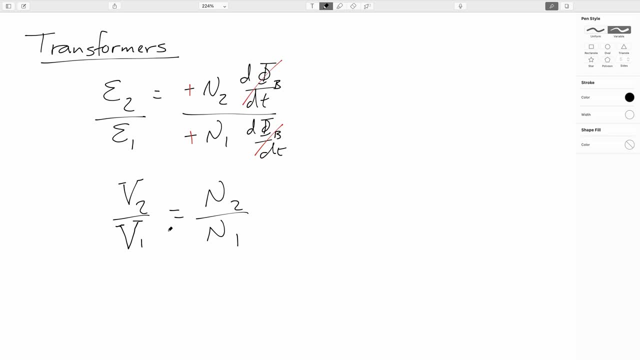 primary, you'll have 1100 volts going out at the secondary. now you can't get something for nothing, so energy has to be conserved. so this means that the rate of power going out of the secondary, the power going out of the secondary, has to be equal to the power going out of the secondary. 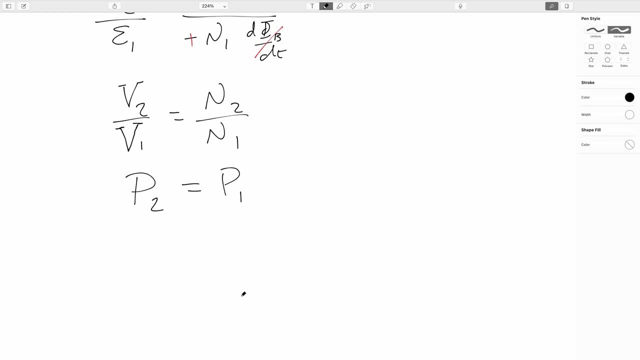 going into the primary. so this will be the current through the secondary times the voltage across the secondary. this will be the current through the primary times the voltage across the primary. so the ratio of the current through the secondary to the current through the primary is equal to the. 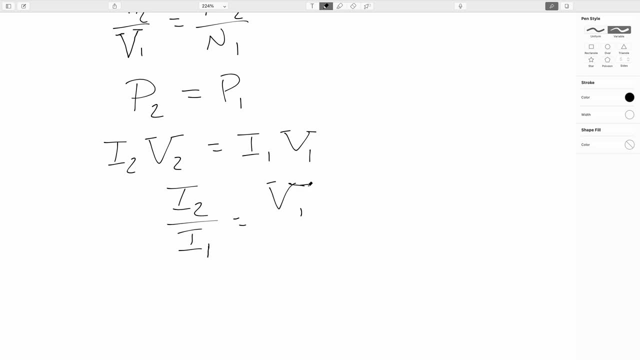 primary is going to be the ratio of the voltage of the primary to the secondary, which we saw was N1 over N2.. So I2 over I1 will equal N1 over N2.. So what this means is if say we have 10 times, 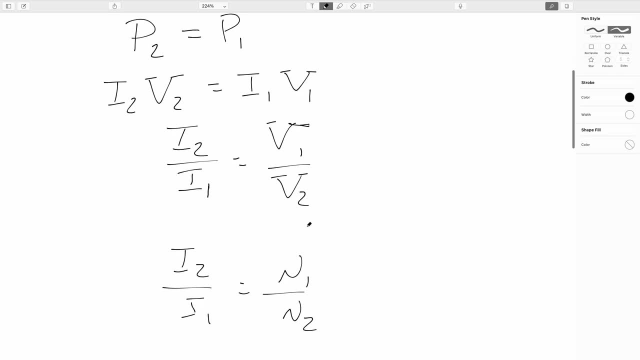 as many windings on the secondary as the primary, the voltage will go up by a factor of 10, but the current will decrease by a power of by a factor of 10.. So in practical application, what that does is it drops the, since the current drops by the. 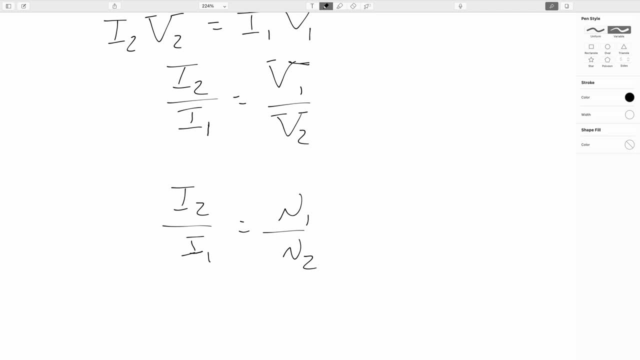 ratio of the windings. the power lost in a transmission line goes as the square of the current times, the resistance of the wire. So say, if you have 10 times as many windings on the secondary as the primary, the current drops by a factor of 10, but the power, the power lost. 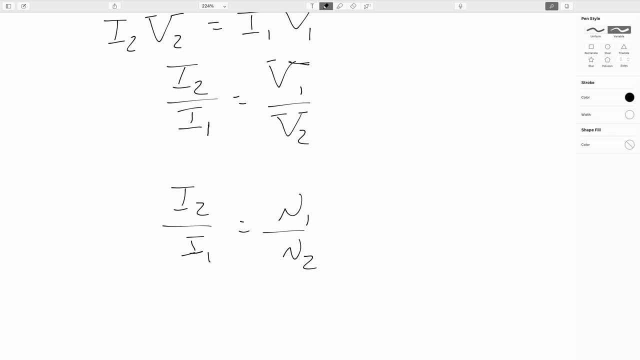 drops by a factor of 100.. And although there are inefficiencies in these what are called step ups, the current drops by a factor of 10, but the power lost drops by a factor of 100.. And although there are inefficiencies in these what are called step ups, the current drops by a factor of 100. 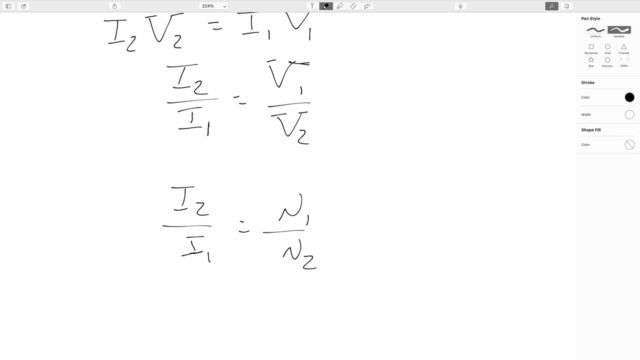 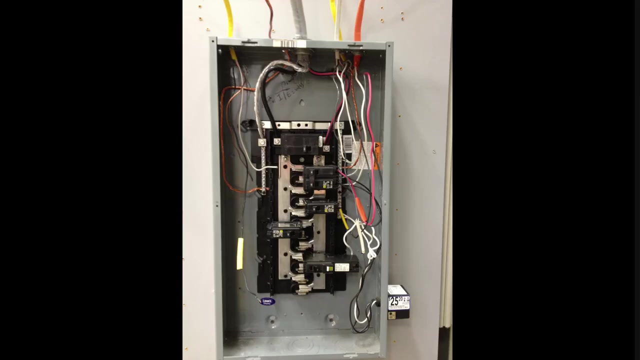 and step down transformers. the savings that you get in transmission line losses is well worth it. So let's think about how the power gets to your house, and we'll start kind of by just working backwards here. So this is a typical North American circuit breaker panel. 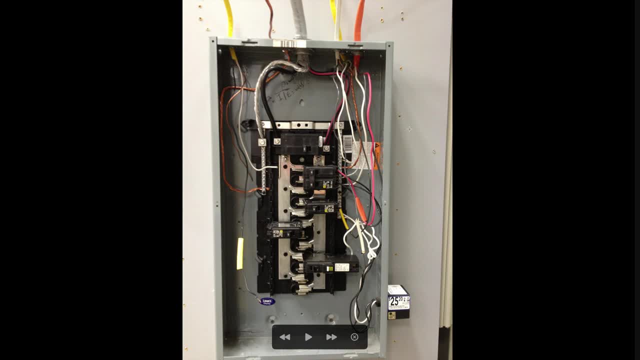 and I will be focusing on what happens in North America, where we use what's called split-phase power distribution to residential areas. so, going into, so, if you remove the protective metal cover in front of your breaker panel, this is what's behind it: This big cable. 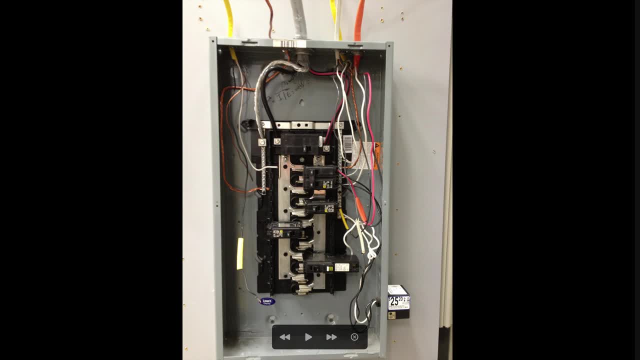 here is what's coming into your power mass from your power mast, This coiled bit of braided wire. here is what's called the neutral. This could also be a white wire. It should stay at zero volts In practice. it might drift a little bit. 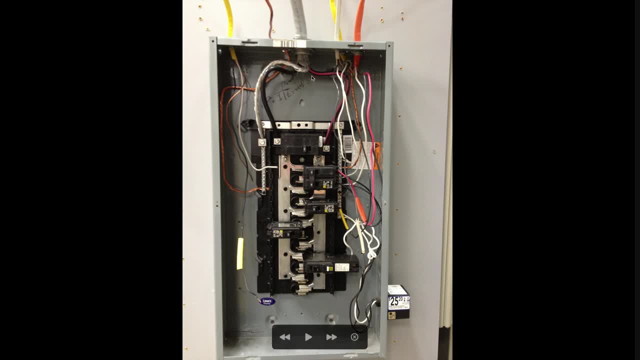 off of that. This black wire and this red wire are both what are called hot wires. This one is known as phase A and this one is known as phase B. So remember: 120 volts AC means that you are oscillating between plus and minus 170. 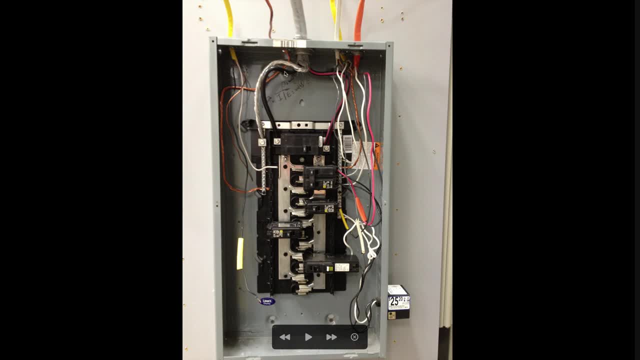 volts. So in phase A this is oscillating between plus 170 and minus 170, and so is phase B. However, they are 180 degrees out of phase, so when the voltage between the black wire and the neutral is plus 170 volts, 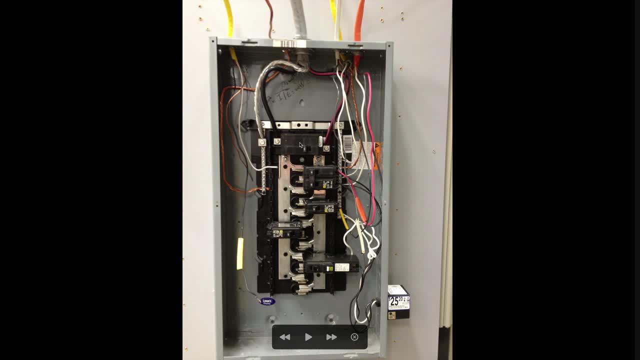 between the red wire and the neutral is minus 170 volts. So the difference is actually 340 volts maximum or 240 volts RMS. So actually a potential difference of 240 volts is delivered into the house. Now this big thing here is the master breaker. 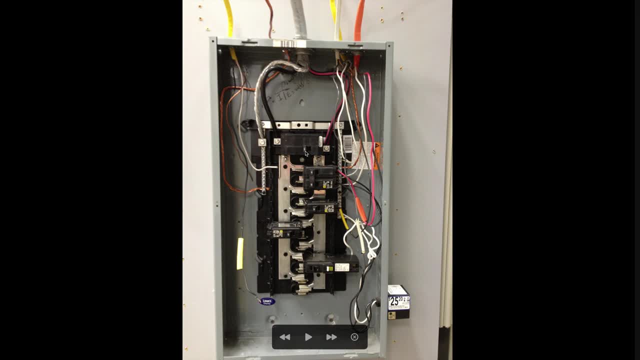 If the current exceeds whatever it's rated for, in this case 100 amps, the master breaker will disconnect both phases from the entire house. Now, going from there, the phase A exits the master breaker and goes on to this bus bar, and phase B also exits the master breaker and goes on to this bus bar here. 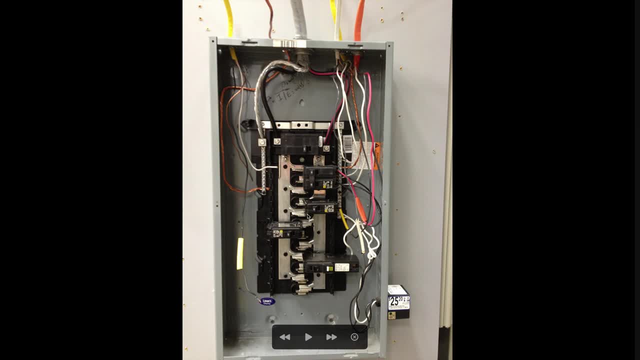 Now you'll notice that the master breaker is disconnected from the house. You'll notice these little fingers coming out of the bus bar. This is so that you can have both 120 and 240 volt service in the house. So for the 120 volt devices, which is pretty much everything except your oven and your dryer. 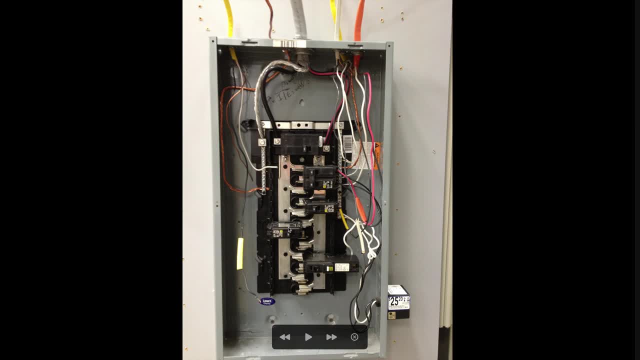 and your air conditioner and your hot water heater, if you have that as electric. This you can see here. This is just sitting on one bus bar. So if the and then the- and you can see a connection is brought off from one of these 120 volt breakers, 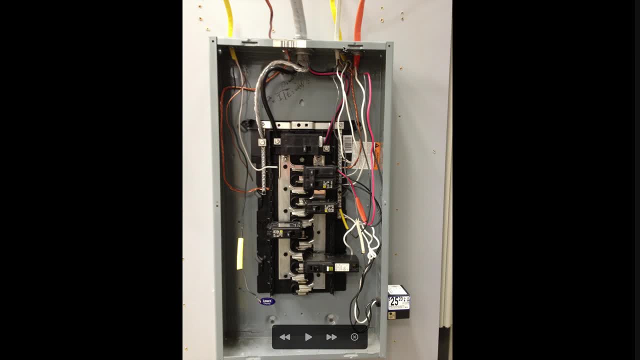 to head off to provide service, along with a neutral. So if it's 120 volts you get either phase A or phase B And a neutral going through the Romex and that connects off to the 120 volt outlets in your house. 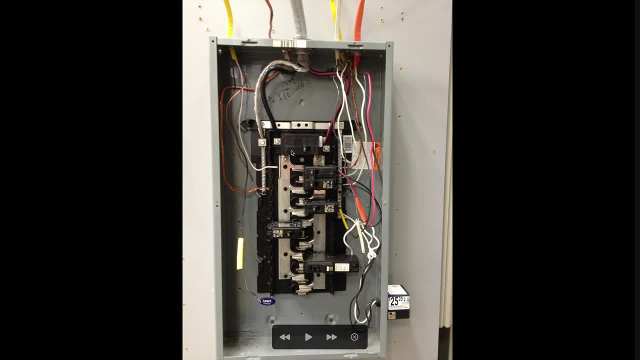 For the 240 volt service, you send three wires: phase A, phase B and the neutral. Now, in more modern houses, there will also be a separate ground. This is because, although the neutral should be at zero volts, it isn't always. 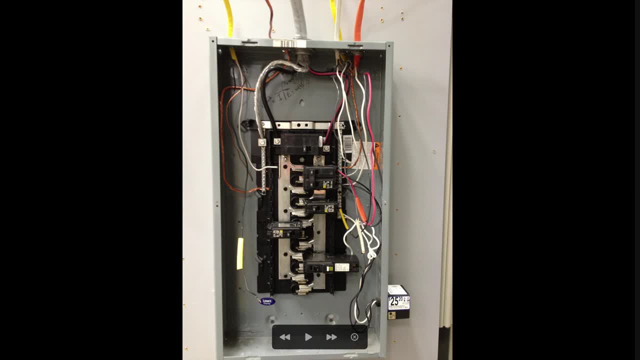 So you can see the neutral. So the neutral's tied in on another bus bar here with a lot of screws And if you look right here, this screw is connected to a copper wire. This copper wire would actually run, actually is going to run, to the outside of the house. 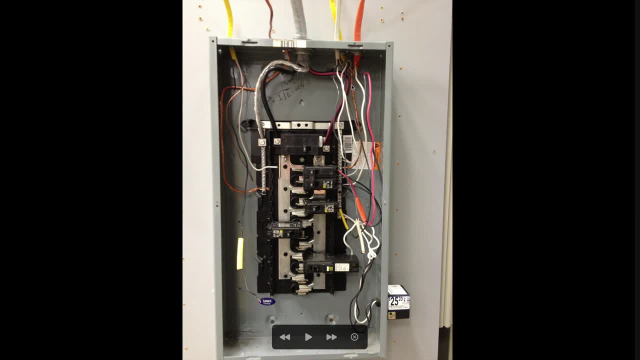 go underground and be attached to a couple of copper stakes buried under the ground. So the idea here is that the amount of charge on the earth at any given time is basically zero, So we can just decide that the earth is zero volts. 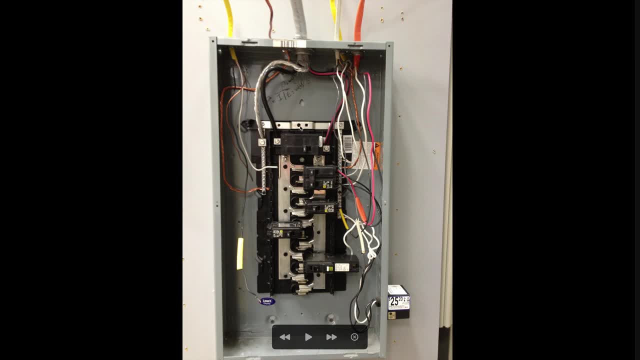 And so this guarantees that the round prong- that the round prong as opposed to the blades in an outlet- are kept at zero volts all the time. The neutral is tied to that, so it should also stay at zero volts, But there can be some problems with that. 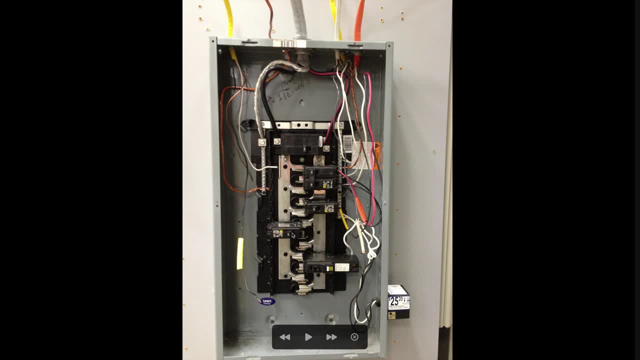 But there can be some problems with that. There can be a little bit of fluctuation. This is because, since you are pulling off of both phase A and phase B, the demand from one side of the house versus some other circuits in the house might not always be perfectly balanced and this can cause a little bit of drift. 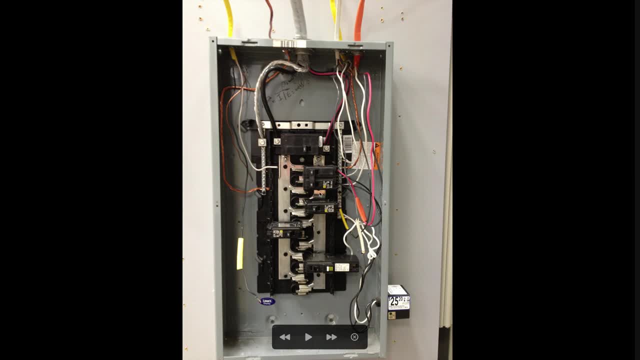 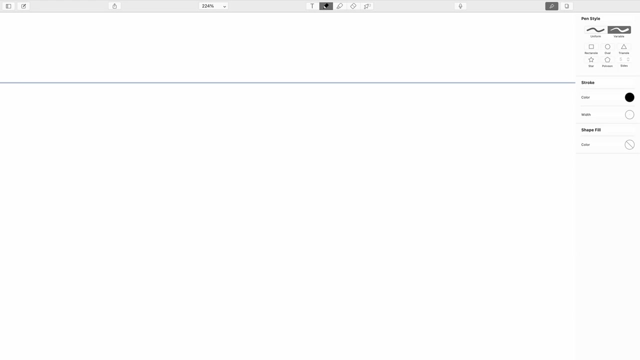 So whenever new circuits are added, electricians have to do calculations to figure out which side of the panel they should add the next circuit on to. So let's see what that looks like when it gets to the plugs in your house. So for the 120-volt plugs, 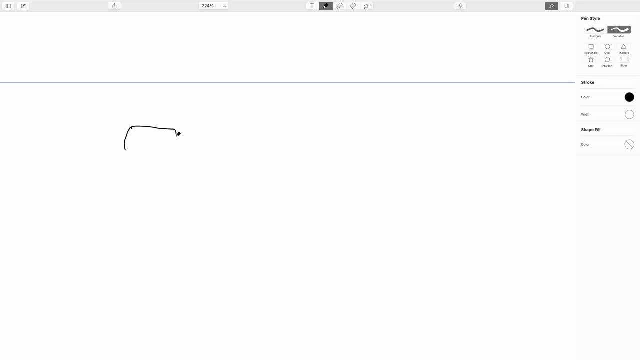 so this is a 120-volt plug. you're going to have a wide blade and a narrow blade and a round prong, like so, And the short blade will be connected to what's called the hot. This is either phase A. 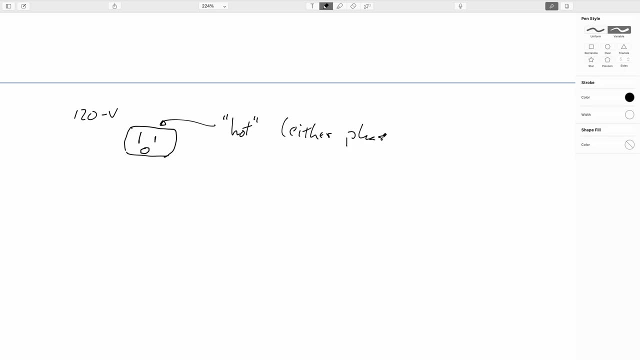 or phase B, And then the wider blade will be connected to the neutral, which should be zero volts, And then the round prong is the ground, which definitely is zero volts. So that's a 120-volt outlet, If it's. 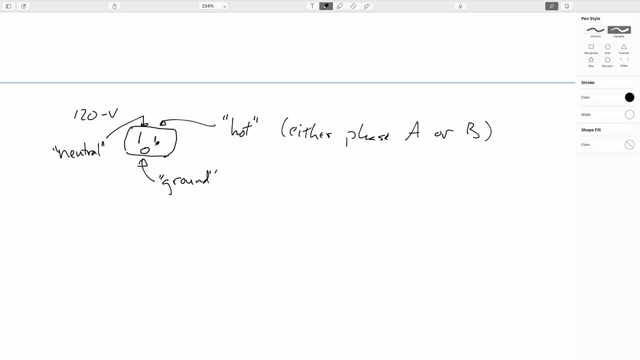 looks like this. it means that the maximum that this outlet can provide is 15 amps. If you see like a little T-shape on one of these, then that means that you can provide up to 20 amps. Okay, so the problem here is that 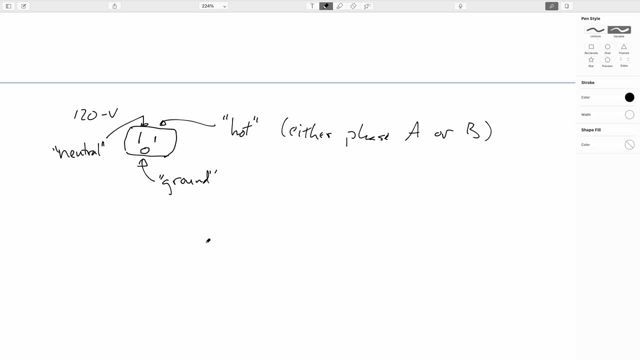 certain very hydrod devices like your oven and your dryer can pull an awful lot of current, And so, again, the resistive law is those who don't have a pressure segregation losses within just the wires in the house can be so high that you run the very serious risk. 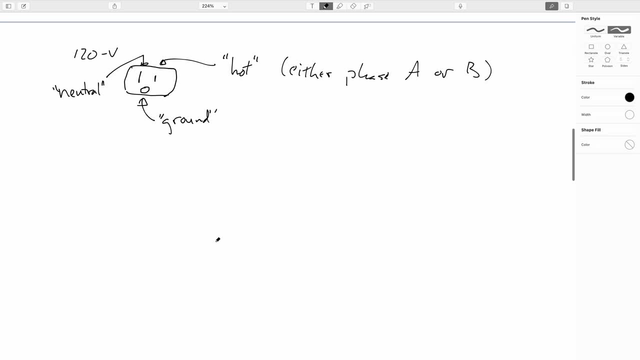 of catching the house on fire. so this is where the 240 volt supply comes in. so your oven plug- which this is also used for from recreational vehicles- will typically look something like this, and this is a much larger plug than the 120 volt plug. so you'll again have a round pin here, which is the ground. 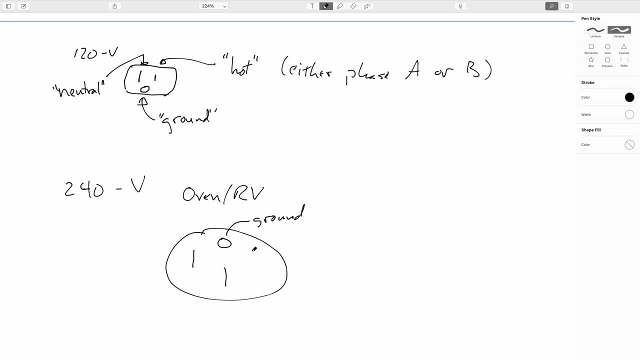 and you'll have three vertical blades like this. this one will. one of these will be phase a, um, so let's say it's that one. this one here will be phase b and then this one here is the neutral. so when you're running the oven, the cal rod in the oven is just connected directly across phase a and phase b. so when this 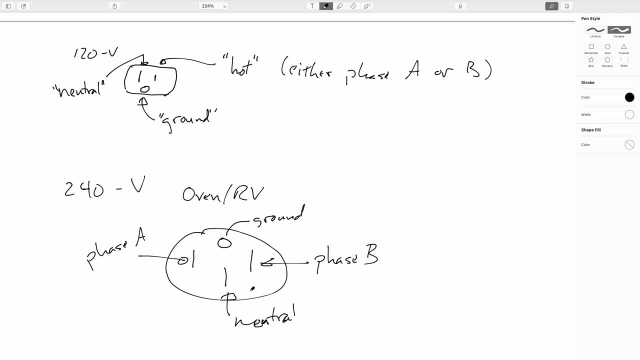 oscillates up to plus 170, this oscillates up to plus 170, and then this oscillates up to plus 170.. it's down to minus 170 for a grand total difference of 340 or 240 volts rms. by having double the voltage available, that means that the oven can pull half the current, which means that 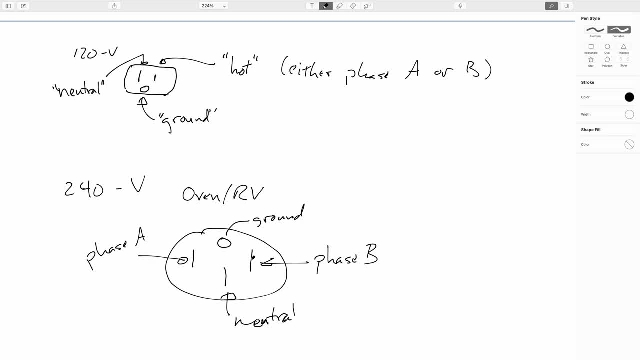 for the same size wire, the rate at which the wire leading to the oven is dissipating heat is dropped by a factor of four. this is enough to um make sure that you don't have to have fire hosed sized wires. okay, i'm exaggerating a bit, but very this means that you don't have 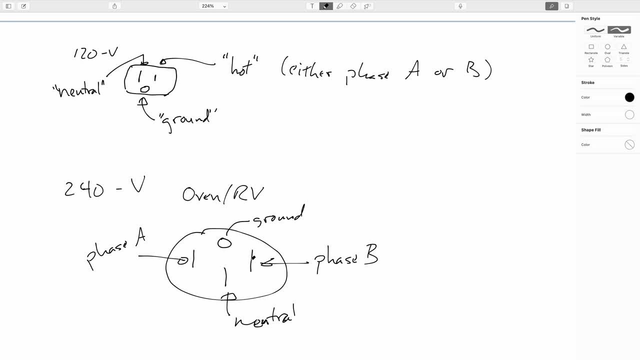 to have very, very fat wires in order to keep the heat losses under control. um, your, your dryer, um. so this is designed to pull a maximum of 50 amps. your dryer is typically rated for 30 amps, and the pin and the plug looks basically the same. um, this is still ground. this is still phase. 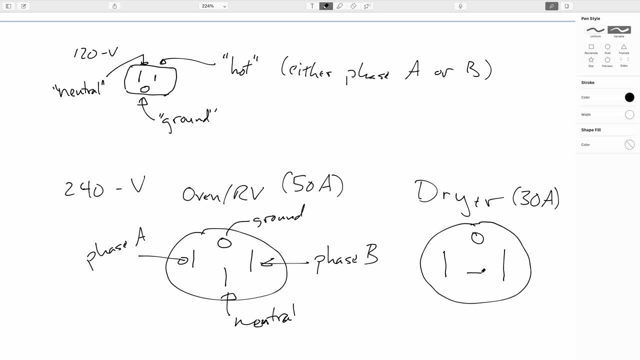 a, this is still phase b. the difference is the neutral, the blade for the neutral, this is still phase a, and then your dryer is still phase b and then you can trailscan. so this is really kind of a case study here. how do we works through this one? because 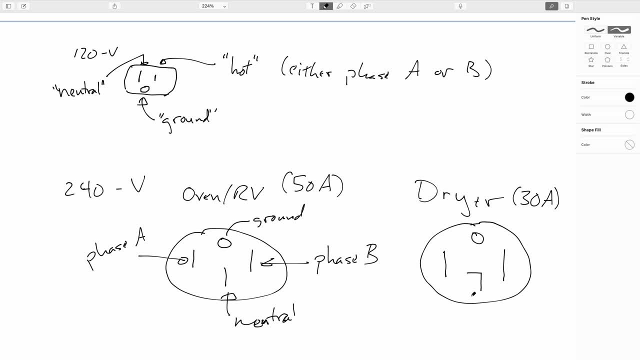 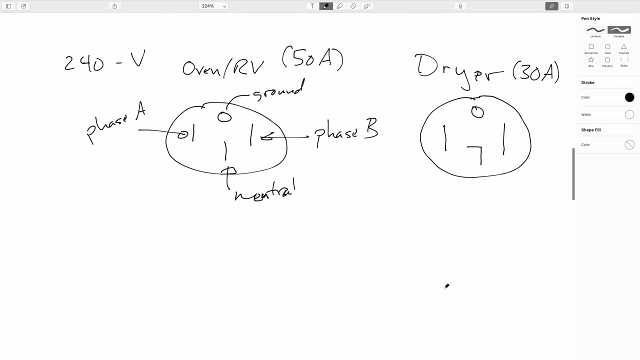 kind of bent into an l shape like that, and this is just to make sure that you don't plug your oven into a dryer outlet, um, because that could be bad. but again it's the same layout: phase a, phase b, neutral. now these are the more modern designs, so this will be for construction since the late 1980s. 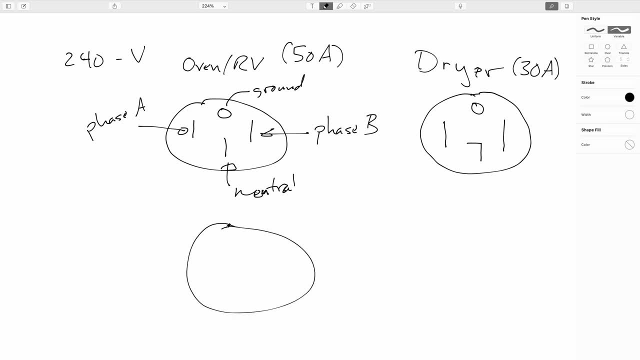 older designs did not have the third prong ground, and so they would have looked like this and like that, and the idea was that, well, of course, the com, the neutral, should be at zero. um, so we'll just assume it is. but here's the thing: the way that the, so the, 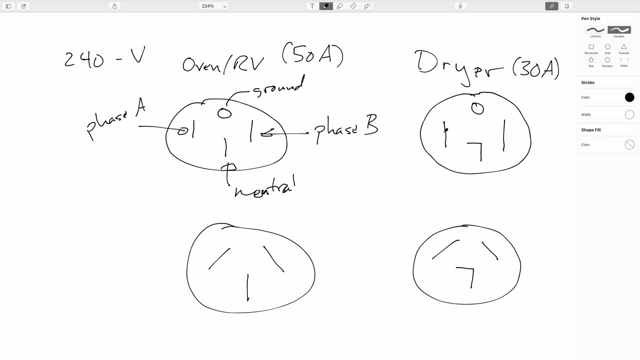 dryer sends phase a, connects the heating element across phase a and phase b, but the motor in the dryer is probably 120 volt motor and so they would just connect the neutral to one of the phases, because this is staying at basically zero. well, this means that you're pulling slightly more. 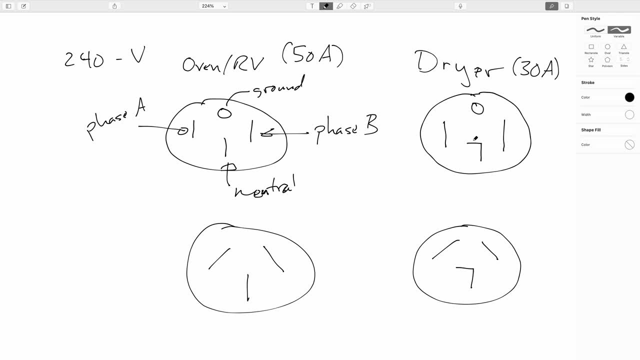 current from one than the other and this will cause a bit of a drift in the voltage here. so if you're down in the basement and also the ground, the chassis- for safety reasons- is um attached to the ground. so here you're making the assumption that it was grounded, but the voltage was actually drifting. 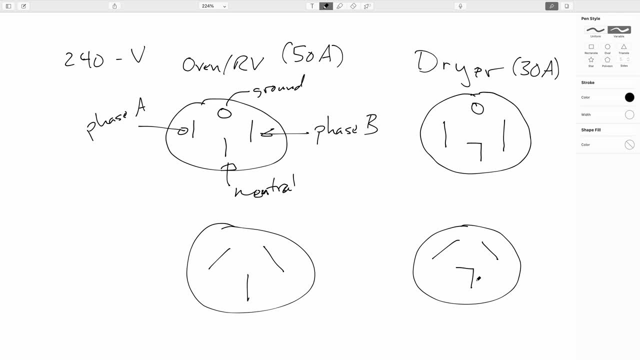 a little bit. and in a basement, in a laundry, you could very well have a wet floor, and if you're standing there with in bare feet in a puddle, that was caused by you doing laundry not very well, um, and then you touched the dryer while it was running there. it could be the case that the 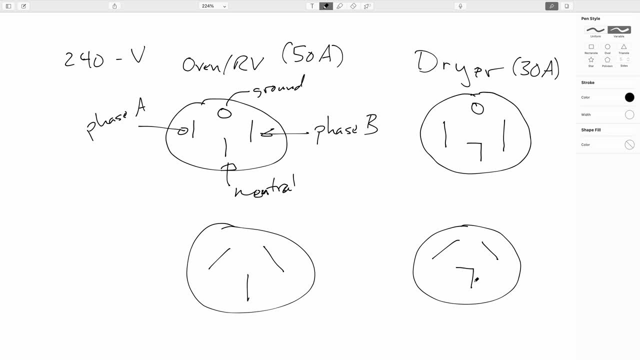 chassis of the ground which is hooked up to this pin could actually be at a few volts and you get a little bit of a zap, and that wasn't a good thing. so, generally speaking, for safety reasons, um, the ground, which is guaranteed to be at zero, came in and now the chassis of the 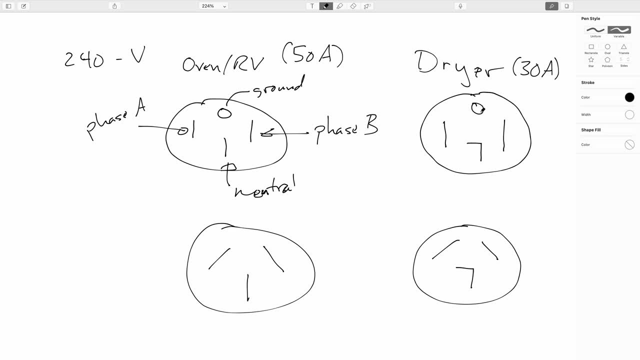 dryer is attached to this pin here. so then, if you touch it while standing in a puddle, you really shouldn't, but if you do it accidentally, this is guaranteed to be at zero volts. the puddle that you're standing in will find you a pathway to ground which is also zero volts. 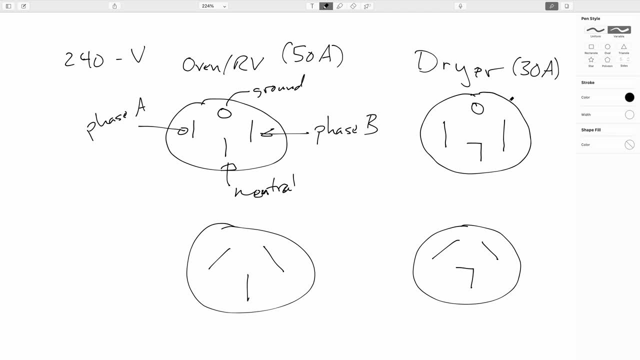 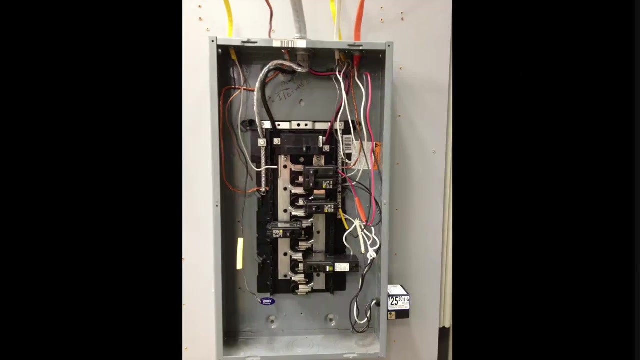 and so you won't pull any current through you, and you won't get a surprise. now, how does it get from? how does it get to your house? well, it turns out that the way power is delivered up to the neighborhood is a thing called three-phase transmission, which i won't really get into too much here. suffice it to say: 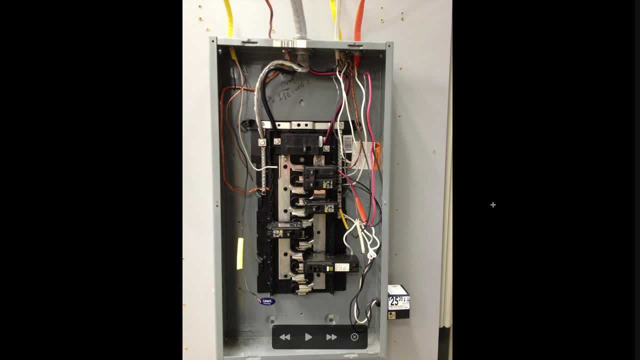 three-phase is what they use in europe and three-phase is delivered straight to the house and there are a lot of advantages to it. but for historic reasons we've got this. but three-phase is delivered straight to the factory because you can build nicer motors with three phase. 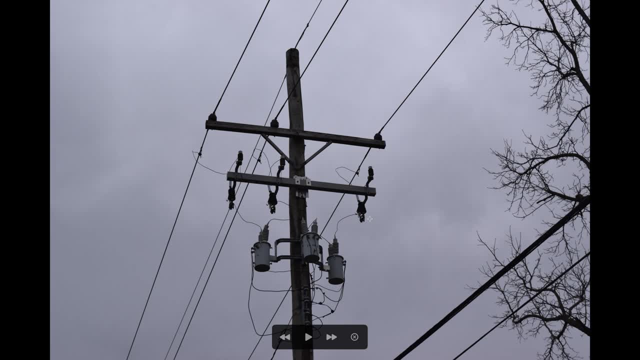 so, anyway, within a few kilometers of your house, you're probably going to see on a utility pole something that looks like this: this is where they are pulling out the three phase that's coming. the three phases are coming from the substation and they're sending phases to individual phases. 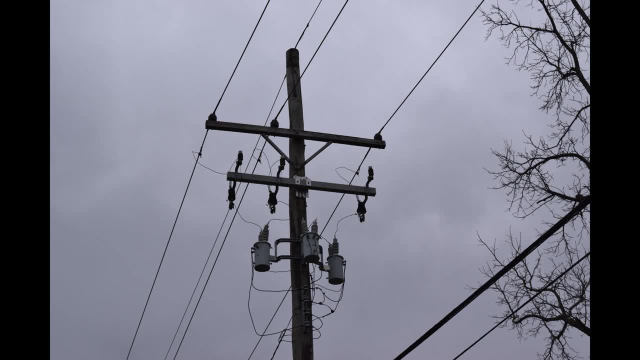 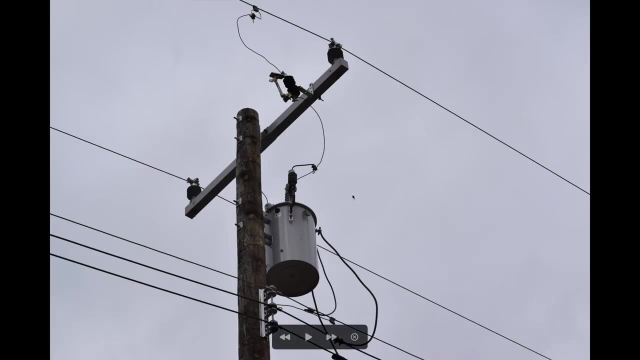 to different neighborhoods in in the area. when you so coming in here, what you've got is: you can see, this is a transformer here. this is attached to one of the phases coming in from the power company and this is at a depends on the power company and how they're doing it. 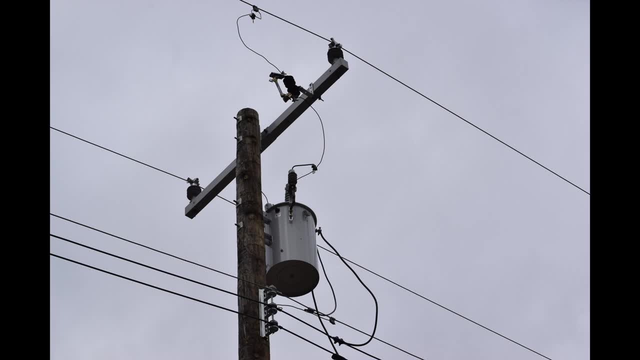 but typically around 7200 volts or so, although it can be higher. um, so then this gets attached along on on one side and then a earth ground line onto the other side to a transformer that's in this can. also in this can is a really big honking fuse, just in case things go. 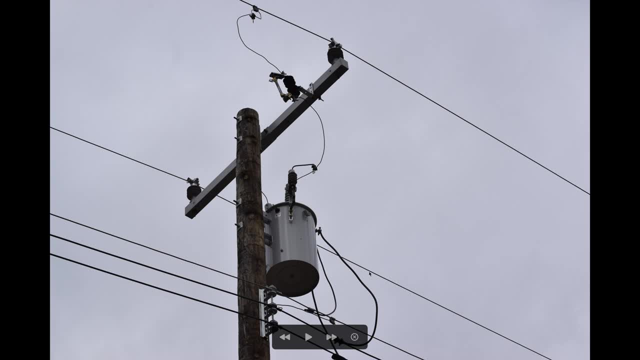 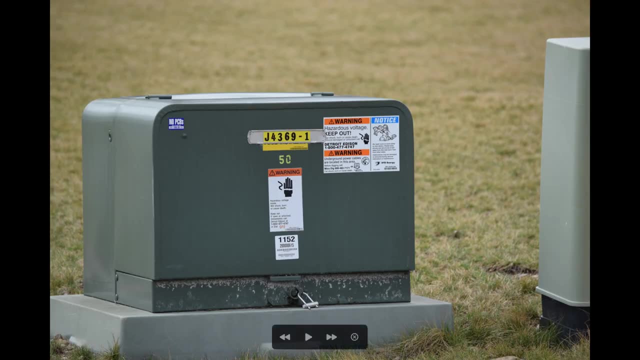 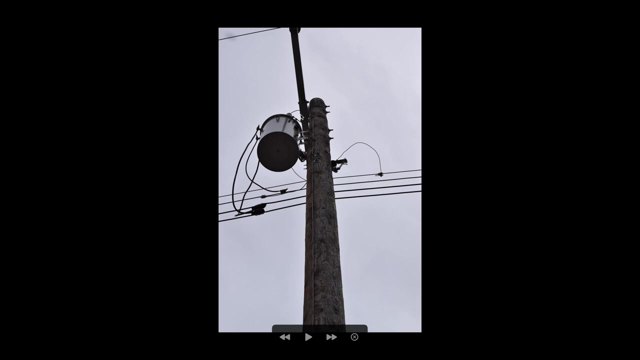 wrong, really bad. um. now, if you are lucky enough to be somewhere where they actually bury the power lines, that will be sitting in typically a green box that looks something like this, but it's the same thing, it's just you can't see the wires. so, anyway, we can see here that the there's wire coming in from one of the phases being provided. 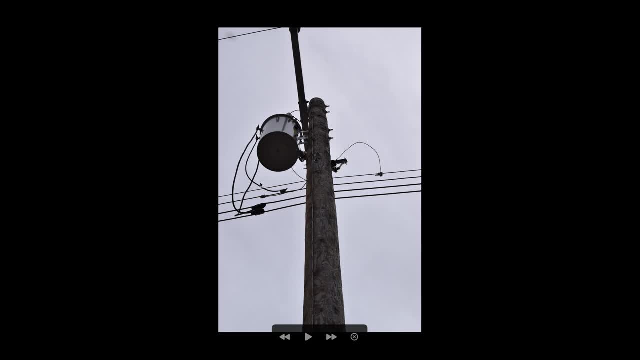 and it goes into the transformer and then you can see, coming out of the transformer are three leads going to three wires. one of these is phase a, one of these is phase b and the other is are neutral. so how do we achieve that? well, see this wire going down here first off. that's the earth ground for. 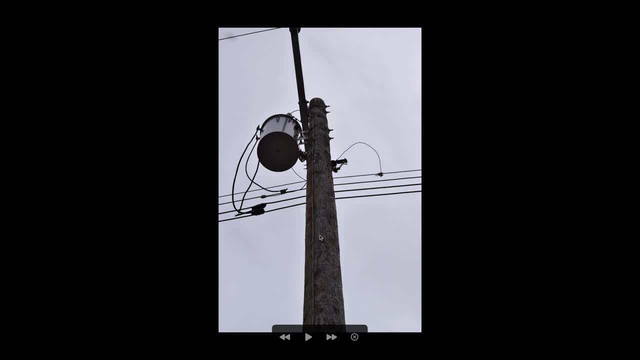 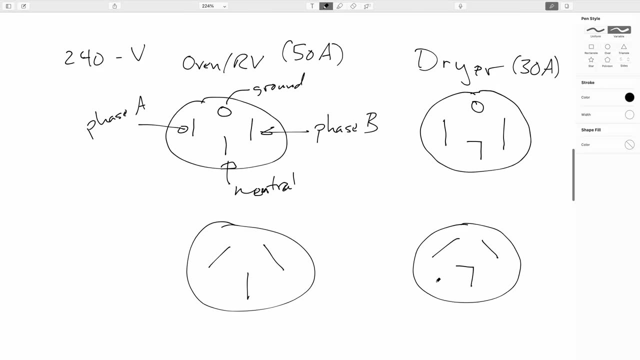 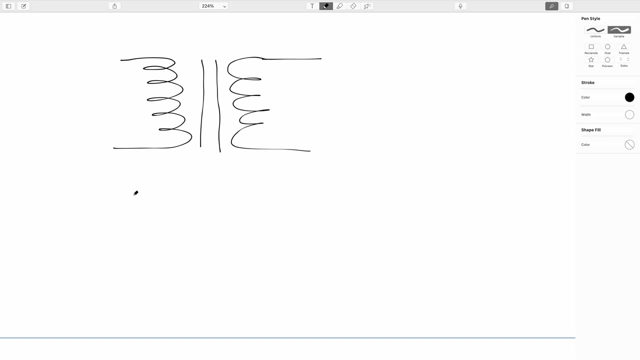 one side of the power transmission, but also coming out of the transformer. um, the transformer is wired up, something is hooked up, something like this. so this is a symbol for a transformer. so these are the two coils in the transformer. let's say this one's the primary. 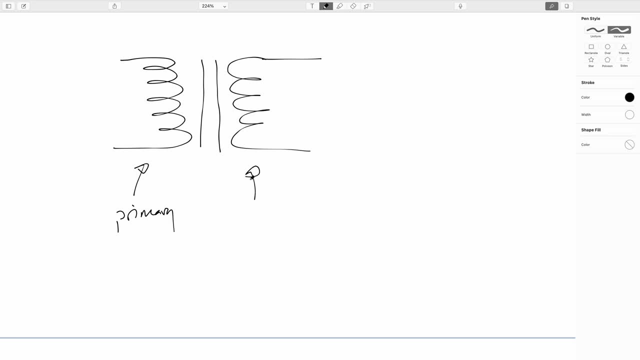 and this one is the secondary um. this pair of lines here means that it's just a magnetic connection, there's no electrical connection. so these two coils share a common magnetic field. so what they do is the primary comes in at about 7 000 volts ish um, and then gets stepped down. 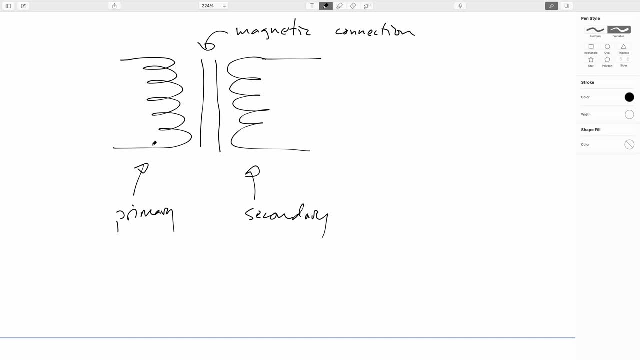 to about 240 volts. if you notice, the wires going in into the transformer are much thinner than the ones going out. this is because when we step down the voltage, we step up the current, so we have to make the wires fatter in order to reduce transmission losses in the line. but then what? 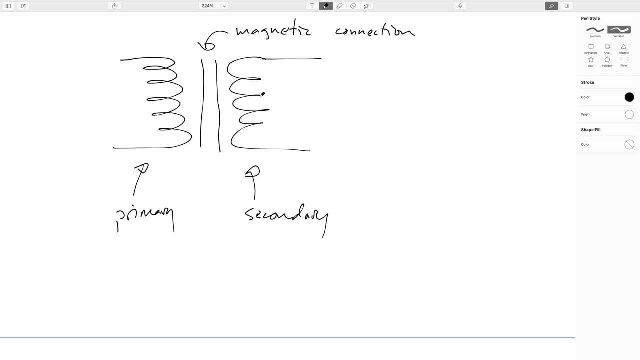 they do to provide the split phase is that there's actually a third connection just tied in somewhere in the middle of the coil, actually at the exact center of the coil, And then this is what gets run down, that wire down the post, going all the way into. 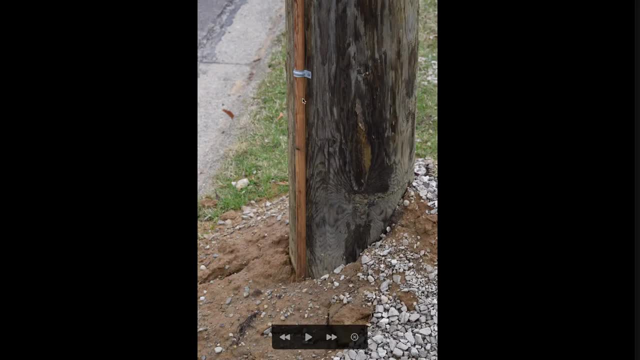 a stake in the earth. There's a little cover here just to make sure people you know, nobody cuts it accidentally or anything like that, but the wires continue to run down the pole and into a stake in the earth. So again guaranteeing that it is at zero volts. 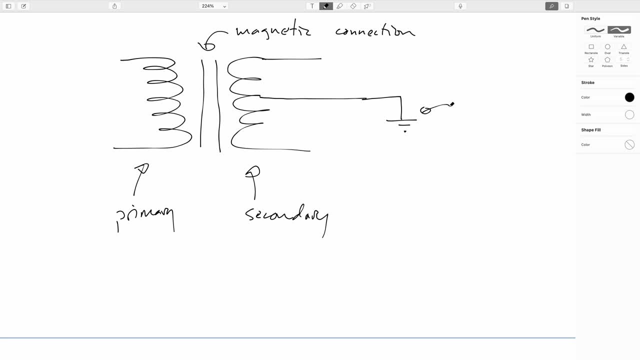 So the symbol for that is this. so that just means ground. So we've set this to be at zero volts, but the difference across these is 240 volts. So that means that there is a 120 volt difference here and a 120 volt difference here. 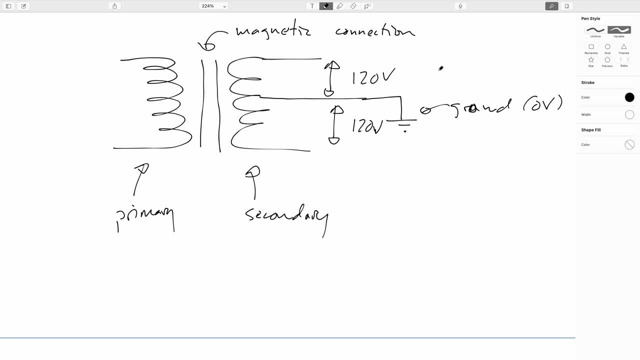 but they will be that the difference across the whole thing will be 240.. So this becomes your phase A and this becomes your phase B. going into the house. All right, but where did it come from there? 7200 volts is still a really high voltage. 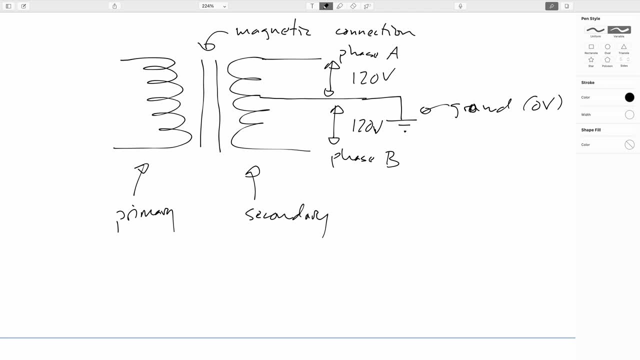 And it's because they can't step it all the way down to 240 from the substation. The runs would be too long, So several, so up to a few kilometers away probably from where you're at, from where these 7200 volt lines are. 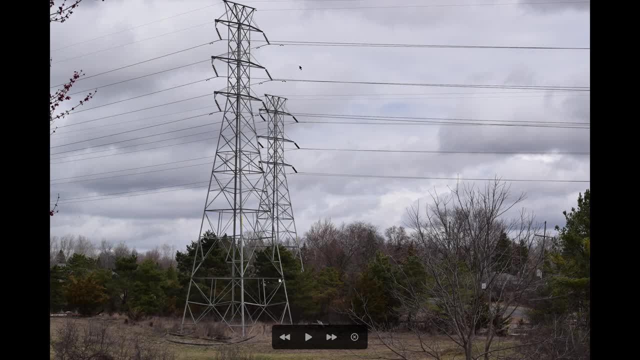 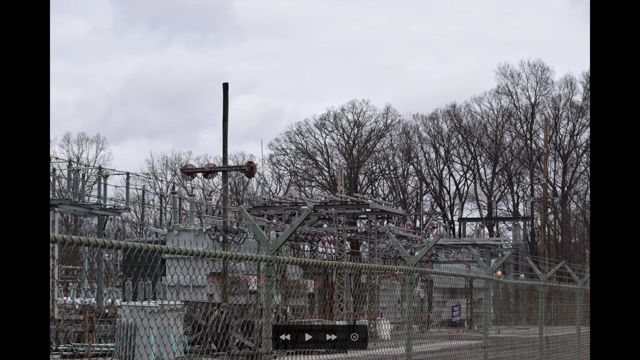 You'll probably see in high tension lines like these, where these could be anywhere on the order of about a half a million volts potential difference, or even higher, And they will go into typically fenced off installations like this because unless you know what you're doing, I mean all these. 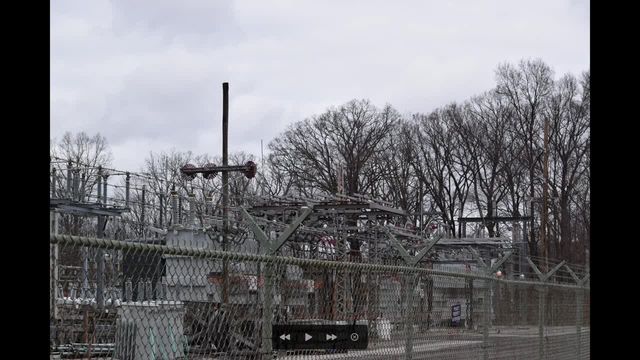 wires that you see here. they're not insulated, they are ridiculous voltages. you touch one of those, not knowing what you're doing, you will fry yourself and you can see these huge boxes there. yeah, those are transformers, um, like, like, right there, um, they are really really big transformers and they're stepping down from the half a million or so. 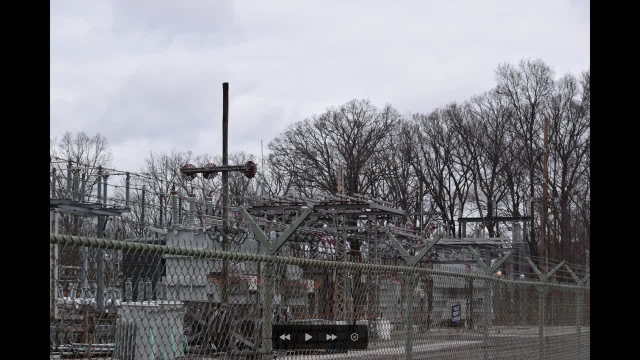 volts down to the 7 000 or so volts, and the current going through the wires will go up in proportion. so on the other end, when you have a power factory, um or power plant, typically they tend to produce electricity at about 10 000 volts or so and then it goes and gets stepped up. 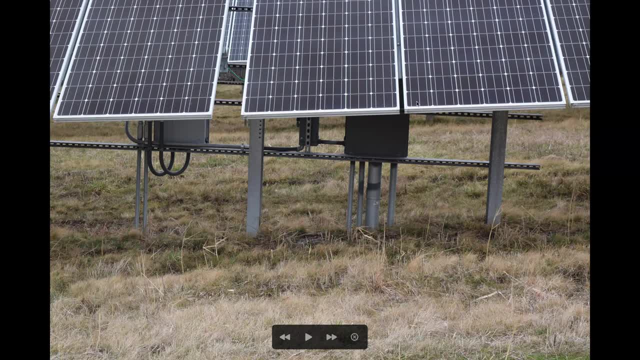 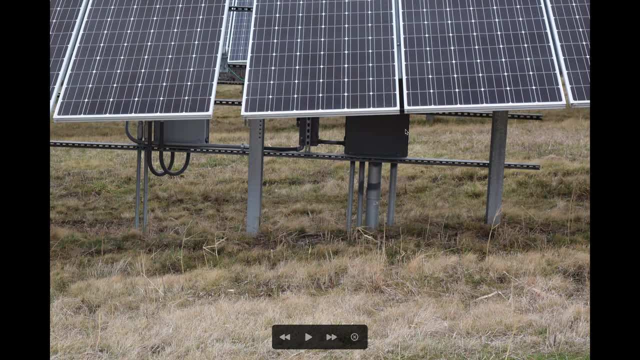 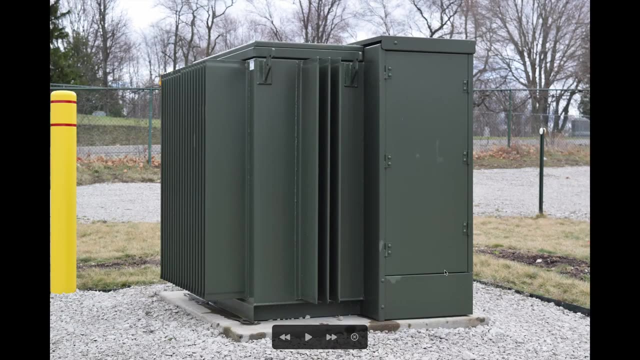 are uniquely dc devices. however, there is. there exists a device called an inverter that will take dc and turn it into ac. the outputs from all these inverters are combined in a giant- basically power panel to make about a 600 volt ac connection in this particular power farm. then this gets stepped. 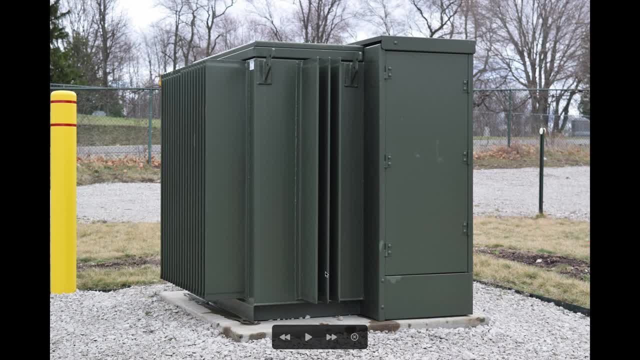 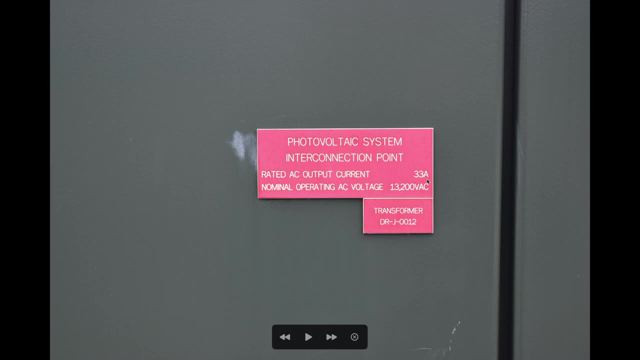 up to, in this case, about 13 000 volts, and this will find its way to some step-up transformer to go into the grid. now take a look at this. so this is at 13 000 volts. the current going through the wires coming out of the transformer is a measly 33 amps, and yet this corresponds to over 400 kilowatts. 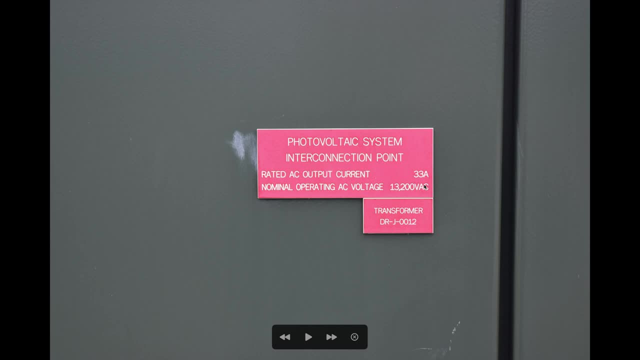 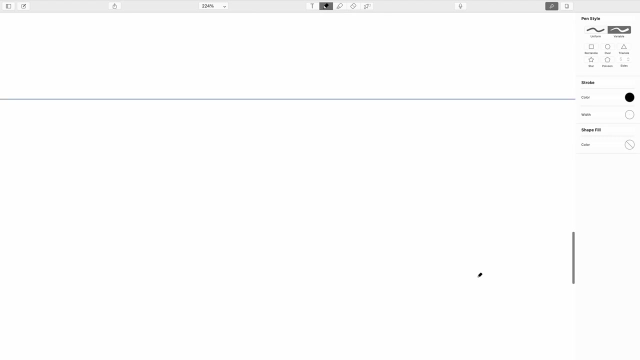 of power being delivered to the neighborhood. so with only 33 amps the um, the uh losses are in the transmission lines are acceptable. now things are changing a bit. i've already mentioned that solar panels are uniquely dc um and so there is some thought that with um, with household uh solar panels, especially if you also have battery storage, which is itself dc, that you might want to start running dc wiring from the solar panel into the battery- in fact this is actually what's done in a lot of sailing vessels- and then you'll again have the use these inverters to get yourself ac for the rest of your devices in the house. 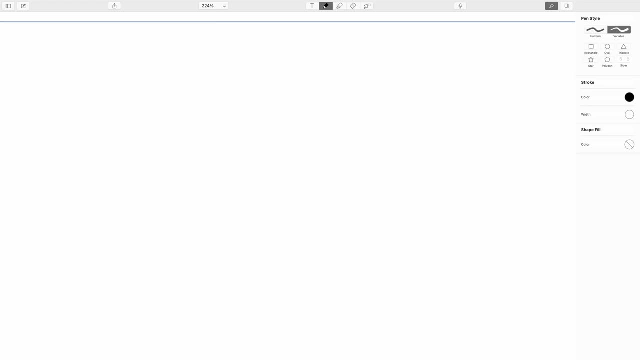 um, the other thing where dc is starting to come back into play is there is sort of a funny effect in ac. if we look at a cross section of wire, it turns out that in ac the closer you are to the outside, to to the outside of the wire, the greater the density of current that gets transmitted. so 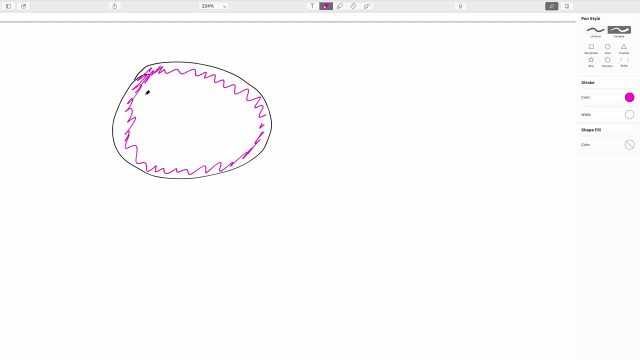 most of the current. this is an effect called skin depth. it's way beyond the scope of this presentation to get into what happens, but suffice it to say that the the bulk of the current gets transmitted on the outside and the amount of current going through to into the interior of 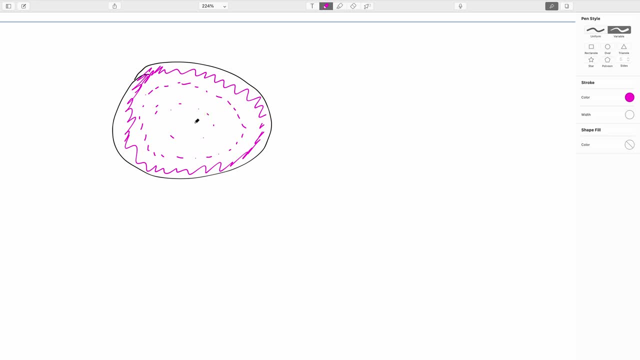 the wire gets less and less, less and less, so with the big transmission lines. you know. just remember, the bigger you make a wire, the less its resistance. transmission lines use very, very big wires but, however, since you're only basically using the outside of it, most transmission lines are actually hollow there. 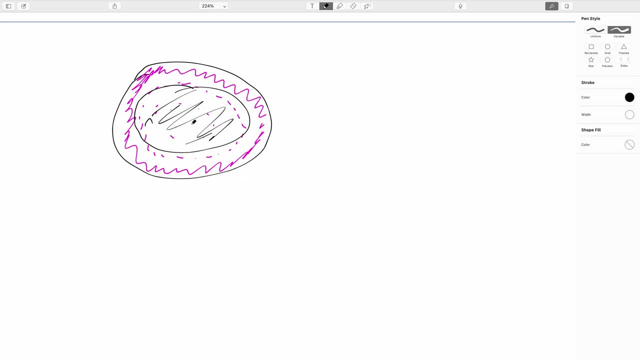 space are stuck inside um, so that the, since you're only using this much of it, this will leave it hollow. to save some electricity, save some uh cost, a lot of cost actually. but this: it turns out that trying to do runs of more than, like, say, a thousand kilometers or so, even at half a million million. 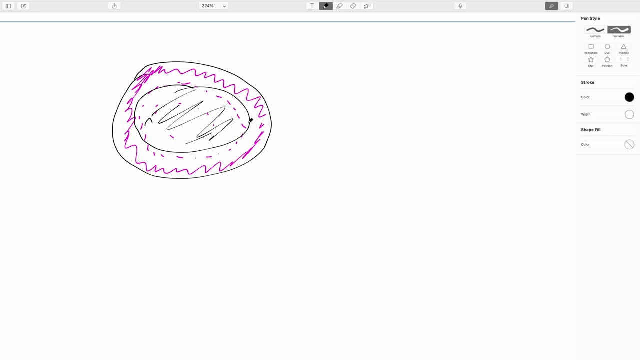 volts, the the loss is become unacceptable. then someone came up with the clever trick: there is a dc? um, there is a device called in a rectifier that will take ac and turn it into dc and so kind of in a funny circle. um, in areas where very long runs are needed for the grid, like say, 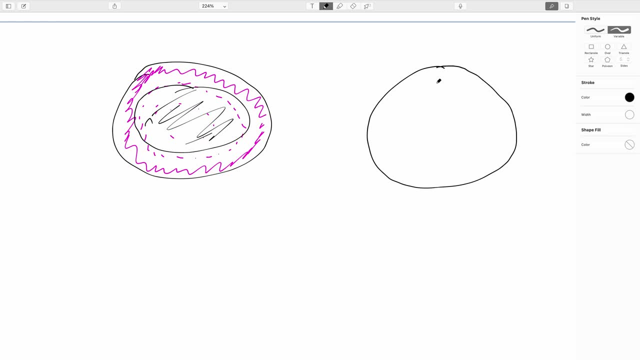 interconnects between between, say, Scotland and continental Europe is one example. There are a few others that are going back to DC. This is because with DC the current is uniformly transmitted through the wire. So although it's a fatter, so you can use a fatter wire. 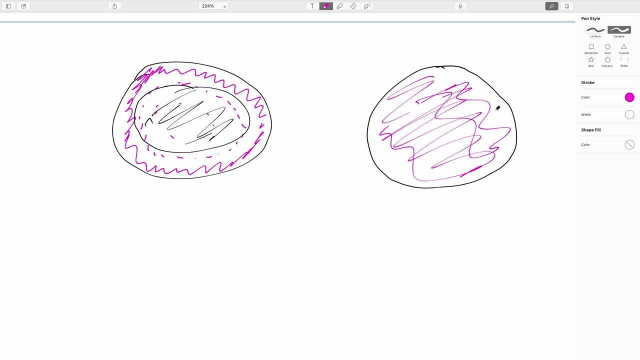 but not only that. since it's distributed uniformly, you can deliver a lot more current through. The trick was being able to make DC inverters that would allow you to go up to a million volts. So again, very low currents going, comparatively speaking. 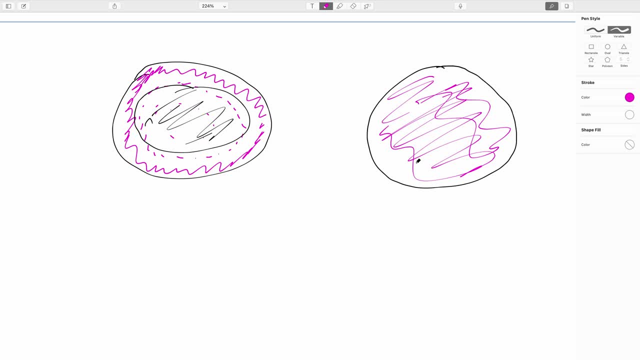 going through these very, very fat wires And by doing this it's become possible to have continent-spanning delivery. This can be really useful, say, in places like Germany, North America, where, in the eastern seaboard- well actually anywhere- the main peak in power demand. 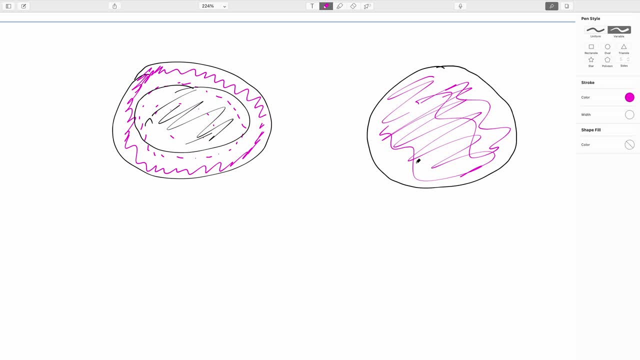 is actually right around about 6 o'clock. That's when everybody's gotten home. They've gone home, They've turned on the TV, They've turned on the oven, They've turned on a whole bunch of devices. That turns out to be the biggest single surge.